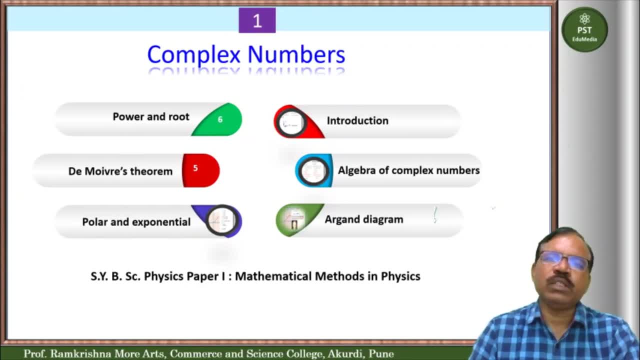 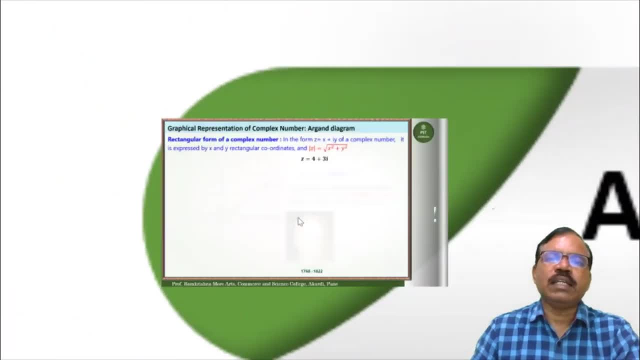 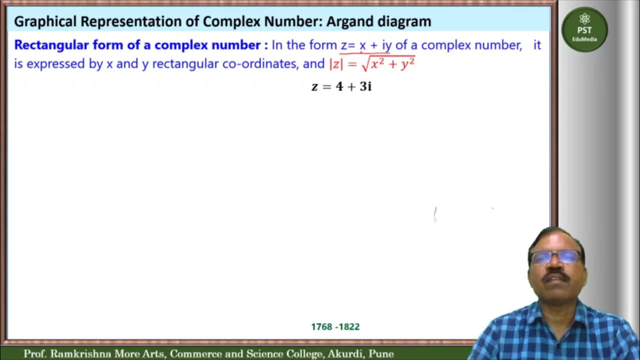 Now in this lecture I will going to explain you graphical representation of complex numbers. So we will go to graphical representation of complex numbers. If we take complex number Z is equal to 0.. Z is equal to x plus iy. This complex number, it is represented by x and y rectangular coordinates on a graph. 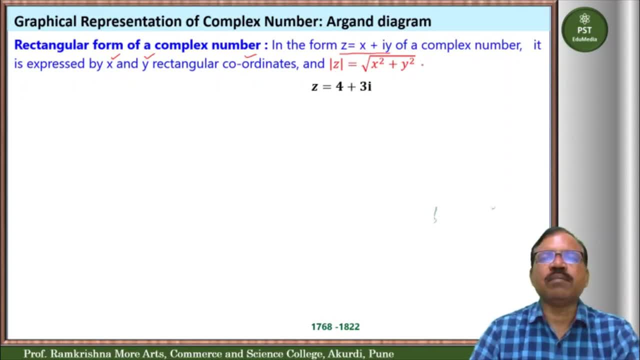 Where modulus of Z is root of x square plus y square. So let us take a graph: Horizontal axis is taken as x axis, that is real axis, And vertical axis is taken as imaginary axis, Also called Z plane. So this one is also called complex plane. 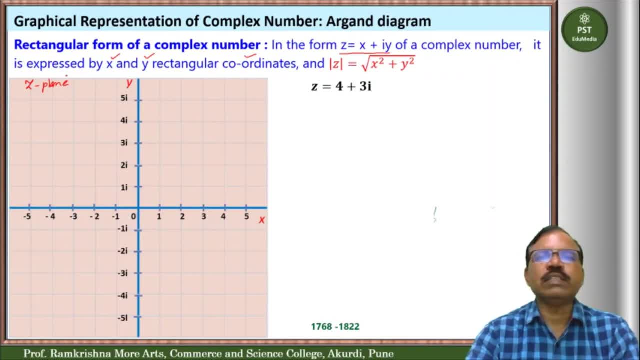 Now how can we represent complex number on this plane? So I have taken example: Z is equal to 4 plus 3i, Where in this complex number x is equal to 4 and y is equal to 3.. So on imaginary axis we take 3i. 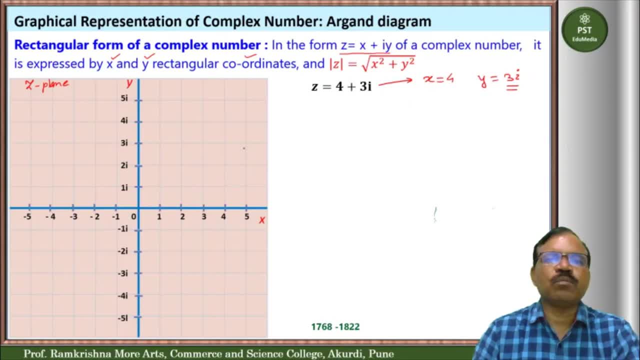 And on real axis we take 4. And we represent a point on the plane. That point is suppose denoted by p And its coordinates are 4 and 3. And if we join line OP, It is actually vector OP. 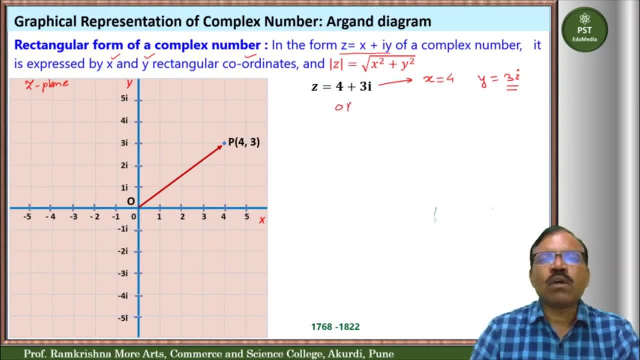 This vector OP represents complex number Z On complex plane. So this is called graphical representation of the complex number. This diagram in this one length OP. It is nothing but magnitude of vector OP. This represents modulus of Z, which is equal to root of x square plus y square. 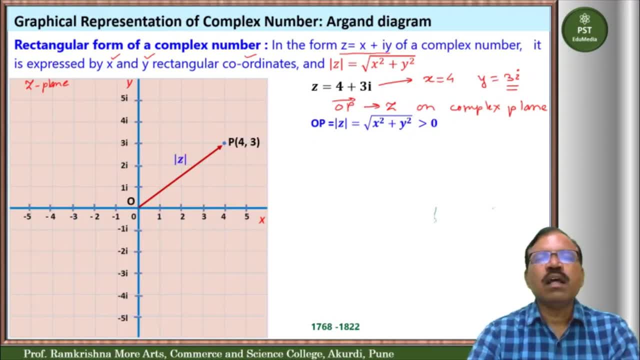 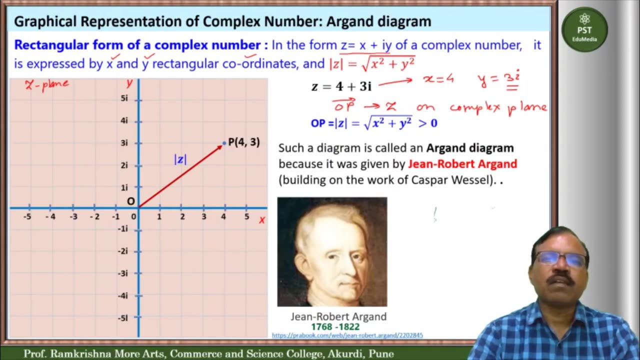 And it is greater than 0. Such a diagram is also called an Argand diagram Because it was given by Jean Robert Argand And it is on the basis of work of Casper Wessel. Now we will use this Argand diagram. 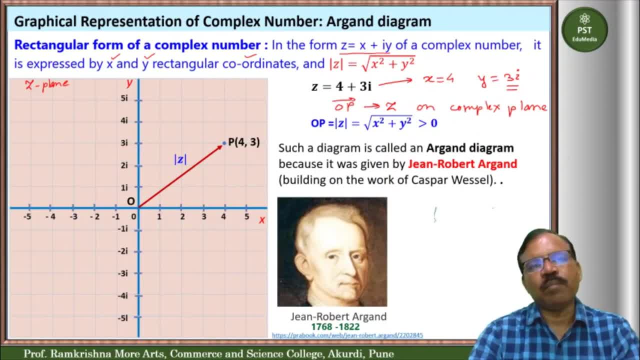 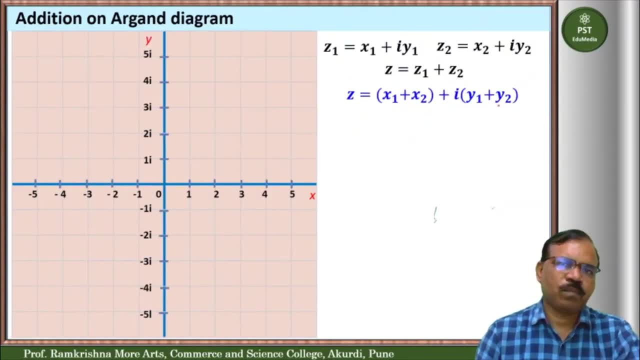 To represent addition of two complex numbers And subtraction of two complex numbers here. So let us take Argand diagram And we have two complex numbers. First one is Z1, with real part x1 and imaginary part y1.. And second complex number is Z2, with x2 as real part and y2 as imaginary part. 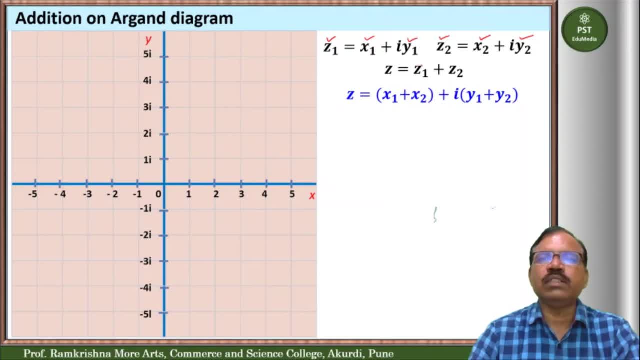 And we have to take addition. So Z is equal to Z1 plus Z2.. Already we have seen algebra of complex numbers In which real part is added in real part And imaginary part is added in imaginary part. So this is also equal to. 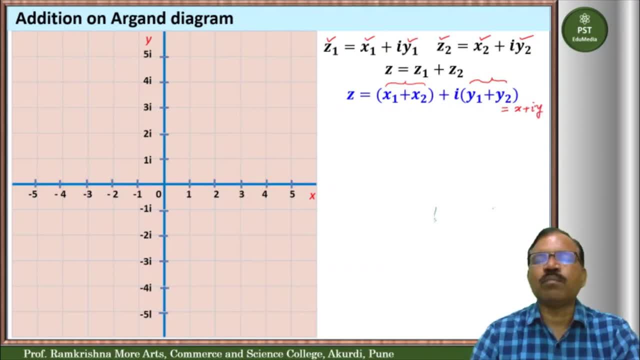 x plus iy. So addition of two complex numbers is again a complex number. Now let us take On Argand diagram. This has Center O supports O, And we take point This is Z1.. So I can write here point P. 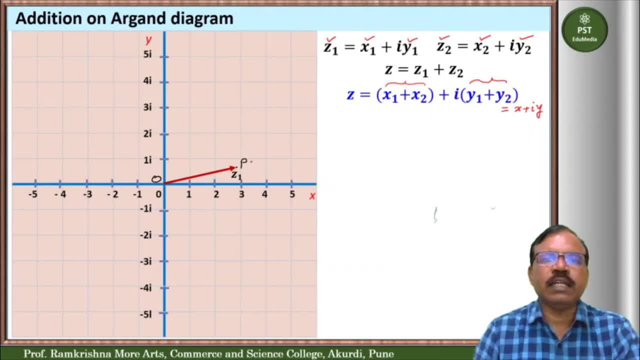 That represents Z1.. By coordinates x1 and y1. Let us take Z2.. That represents By vector Oq, With coordinates x2 and y2.. Now we have to take addition of these, Since here Op vector. 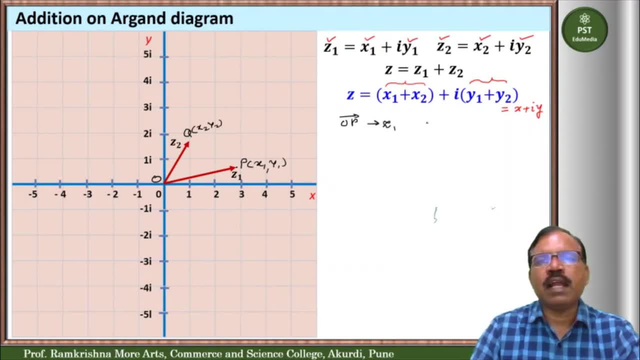 Represents complex number Z1. And Oq vector Represents complex number Z2. So we can take vector addition. So how can we take vector addition? So We take vector Parallel to Oq And start from Tip of Op. 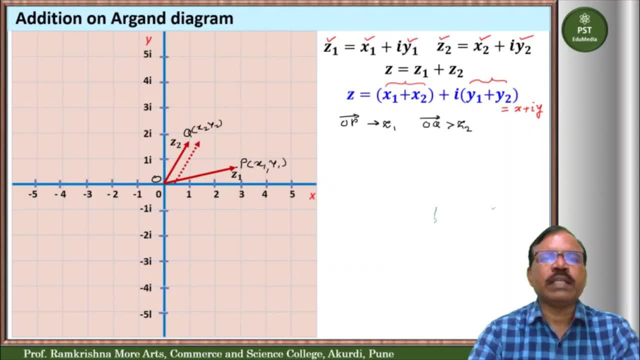 That is from point Op. So we can do like this. Then we take Vector Parallel to Op And start from Point Q, So we get a parallelogram And this diagonal of parallelogram It is, I can call this as: 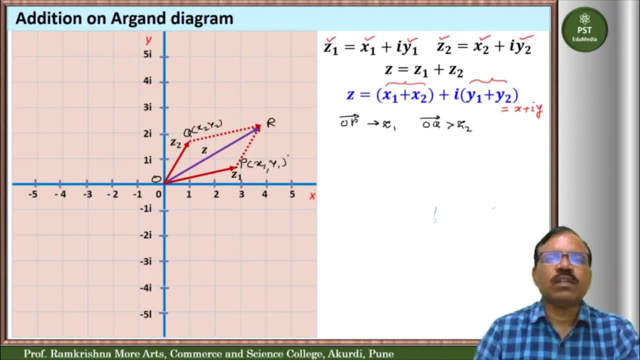 Or So Vector, Or It represents complex number Z, Which is Z1 plus Z2.. Z1 plus Z2.. That is addition of two complex, Complex numbers. Now If we see here Modulus of Z1.. 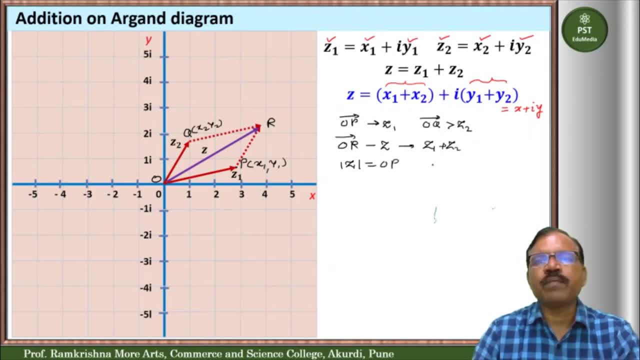 It is Op, Magnitude Op And modulus of Z2.. It is Modulus Oq And if we take modulus of Z, That is Or Now we know Vectorially, And Or Vectorially, Or 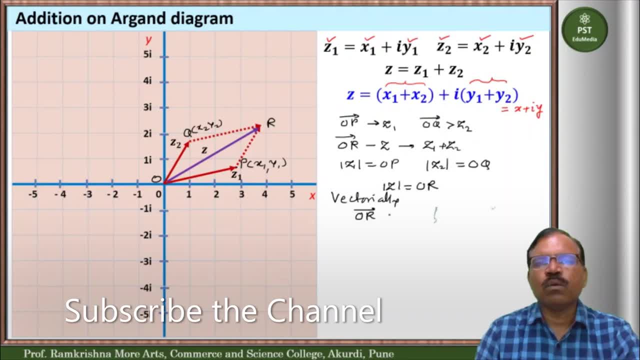 Is equal to Op Vector Plus Oq Vector. But if we see In this diagram Vector diagram, You will observe that Or Magnitude Is not Equal to Op Magnitude Plus Oq. 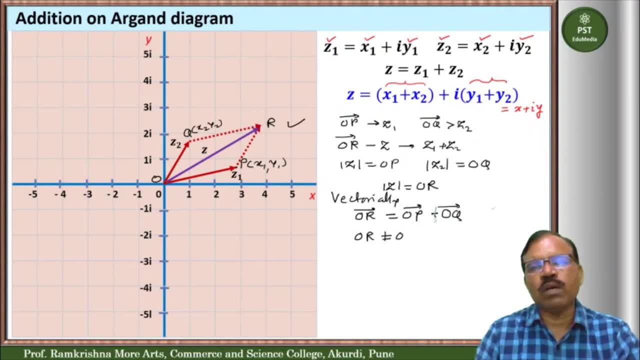 Magnitude. In this Diagram, Vector diagram, You will observe that Or Magnitude Is not In fact, Or It is Less than This Op Plus Oq- Now Here- Or Vector. 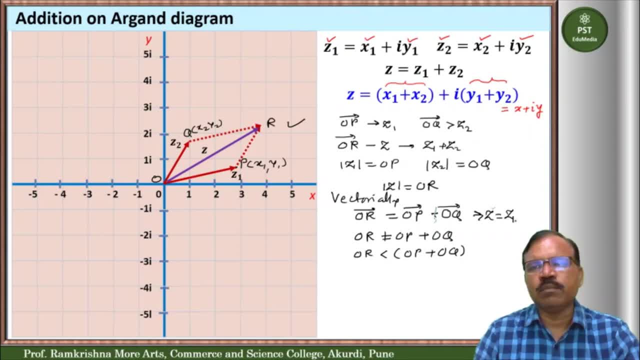 Is equal to Op Vector Plus Oq Vector. This Represents Z Is equal to Z1. Plus Z2.. But if we take Or Or, It is Less than This. But 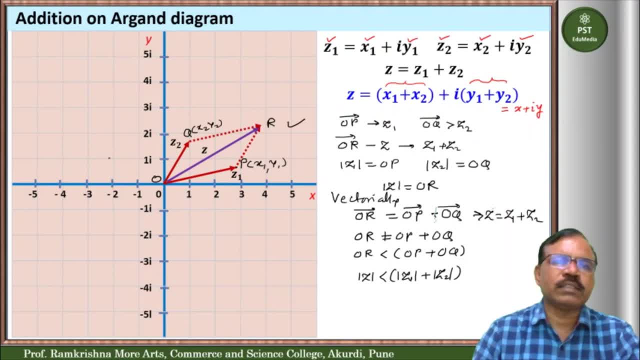 Suppose We have Two Hectors. Suppose This Is First Complex Number And If You Take Second Complex Number On The Same Line, This Is Second Complex. 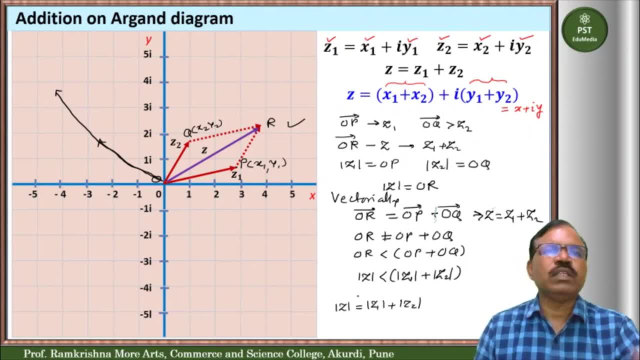 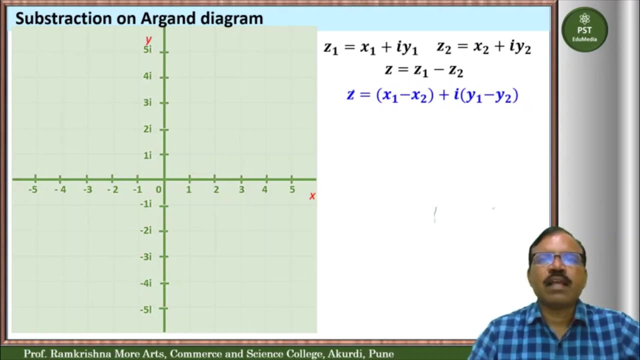 Number On The Same Line. So In This Way We Can Represent Addition Of Two Complex Numbers Using Ergon Diagram. Now We Will Go To. 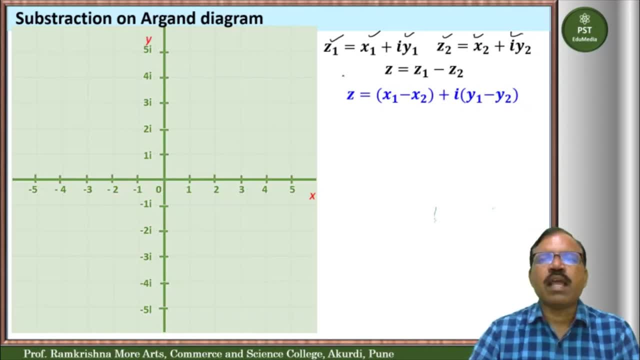 Subtraction Of Complex Numbers On The Algebra Of Complex Numbers, In Which, In Subtraction, Real Part Is Subtracted From Real Part And Imaginary Part. 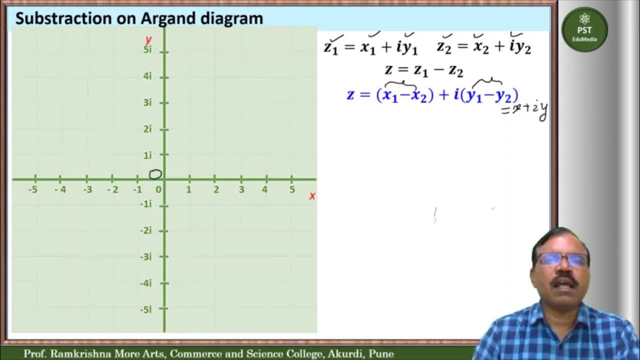 Is Subtracted From Imaginary Part, So We Get This As That Is Z1.. Represented By Vector Op. So Op Vector Represents Complex Number Z1.. 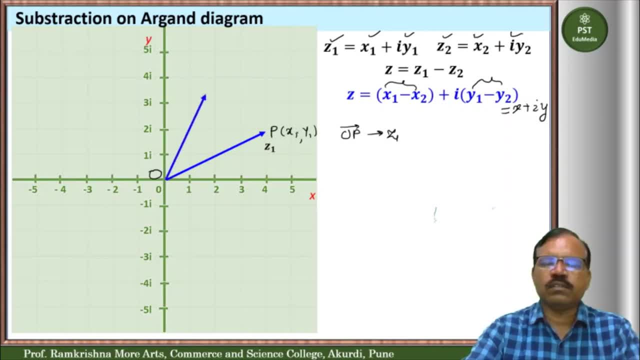 So Coordinates Of This Point: Pr X1., Y1.. Now Let Us Take Z2.. It Is Represents Complex Number Z2.. Now We Have To Take: 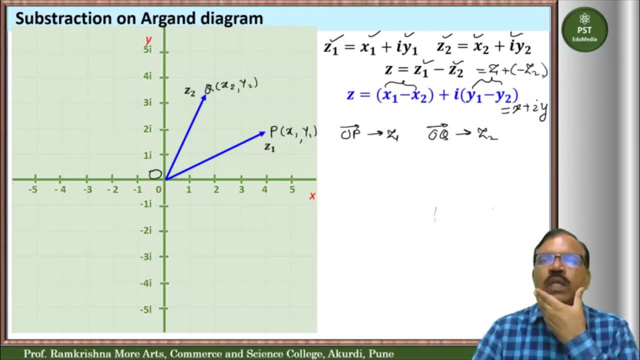 Subtraction. So This Subtraction I Can Write Z1. Plus In Bracket, Minus Z2. So I Have To Reverse Direction Of Z1. So O. 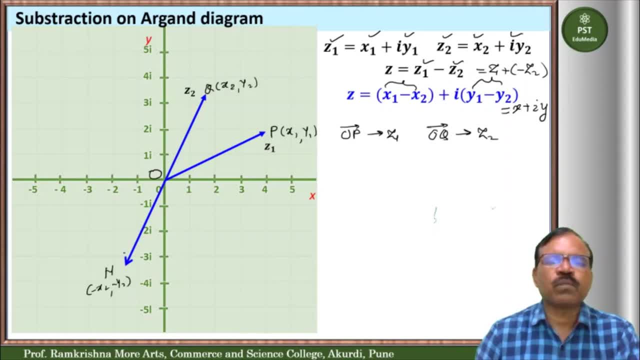 N Has Coordinates Minus X2.. Minus Y2.. Now From O, N And Op We Can Draw Parallelogram Of Vectors. So Here We. 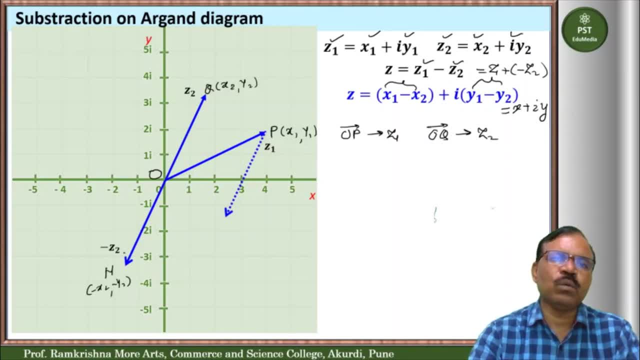 Take Vector Parallel To Z1. And Start From N, So We Get Parallelogram And Then This Is Diagonal Of Parallelogram. We Can: 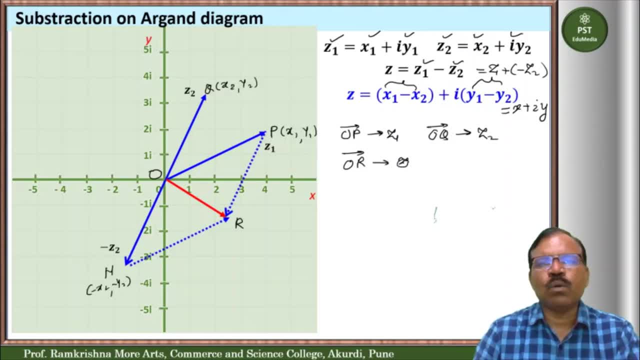 Write This Point As R, So O R Vector Represents Complex Number. N Is Equal To Minus Op, So I Can Write O R Is: